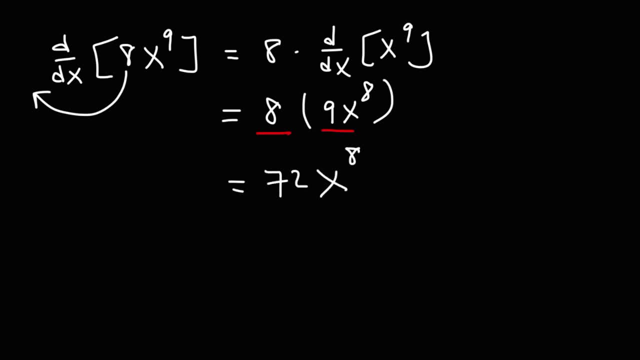 9 times 9 is 72. So that's the answer for this example. So let's say, if we want to find the derivative of 5x to the sixth, It's going to be 5 times the derivative of x to the sixth power, which is 6x to the fifth power. 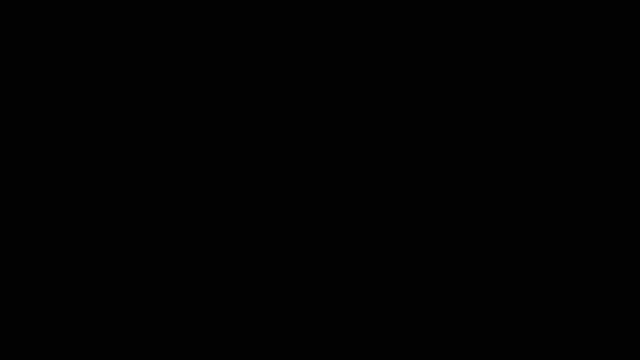 And we're going to get 30x to the fifth. Now what if we want to find the derivative of, let's say, 7x? What's the answer for that one? Well, keep in mind, this is x to the first power. 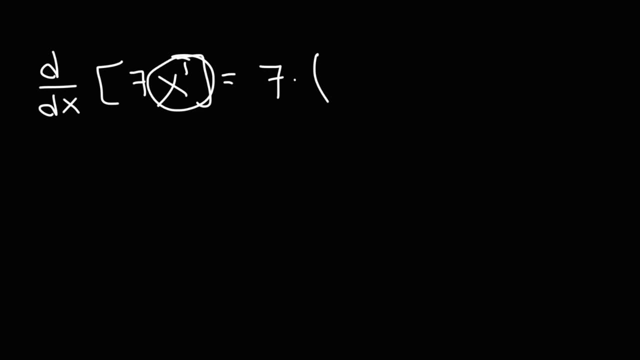 So it's going to be 7 times the derivative of x to the first power, which is 1x to the zero power, And anything raised to the zero power is 1.. So the answer is just 7.. So the derivative of 5x is simply 5.. 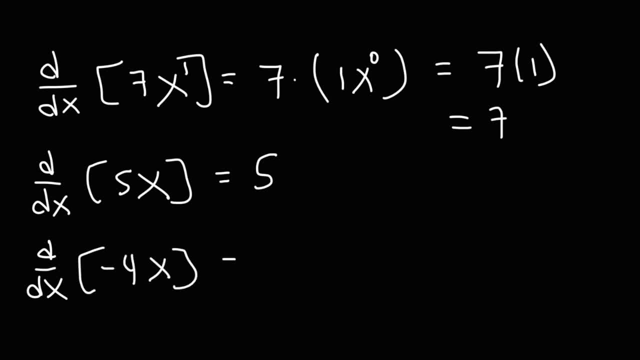 The derivative of negative 4x is simply 5x, So the answer is simply negative 4, following that same pattern. Now, the last thing you need to be familiar with is that the derivative of a constant is 0.. So the derivative of, let's say, negative 6, that's going to be 0. 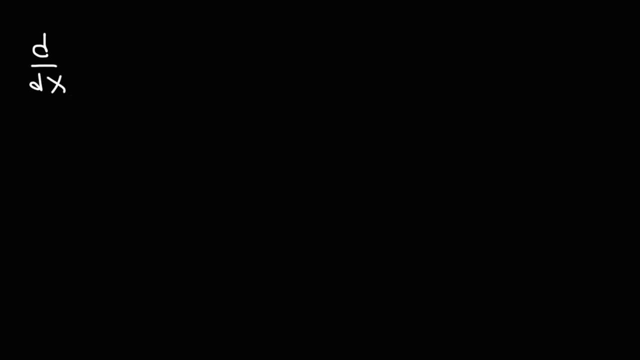 So, now that we had a quick review of some of the basic stuff, let's go over finding the derivative of a fraction. So let's say we want to find the derivative of x over 9. How can we do this? Well, it helps if you rewrite the fraction. 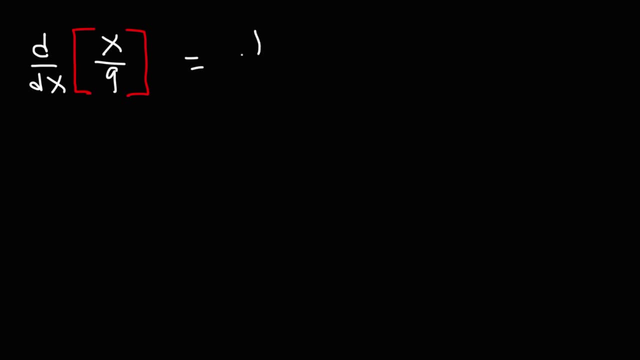 This is the same as the 9 is a constant, so you could say this is the same as 1 over 9 times the derivative of x, Because 1 over 9 times x is x over 9. And the derivative of x is simply 1.. 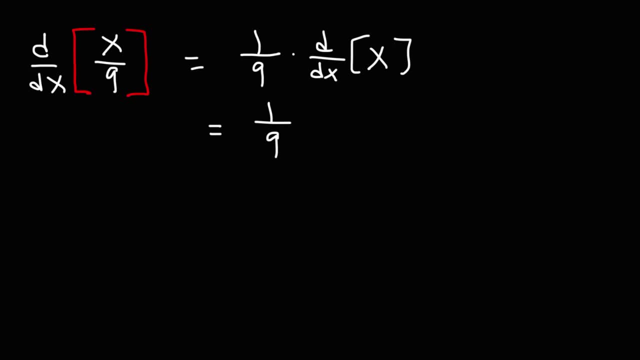 Keep in mind: the derivative of 5x is 5,, 2x is 2,, 1x is 1.. So the answer for this example, it's simply 1 over 9.. Now, what about this one? What is the derivative of 4x over 7?? 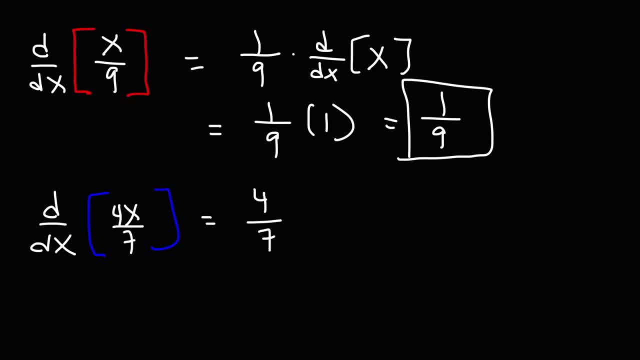 So this is the same as 4 over 7 times the derivative of x, So it's just 4 over 7 times 1, or simply 4 over 7.. So that's what you can do if x is in the numerator. 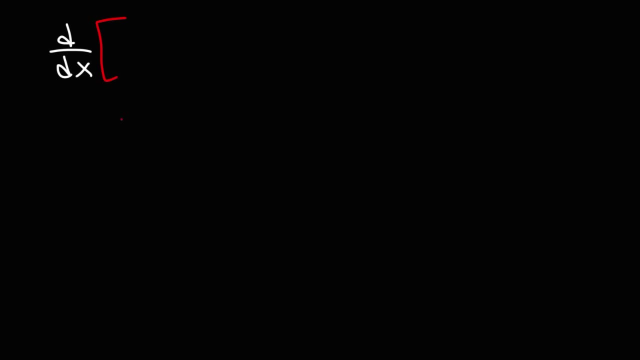 But what if x is in the denominator of the fraction? Let's say we have the derivative of 8 over x. Well, in this case the situation is different. If you see this, what you need to do is you need to rewrite the expression. 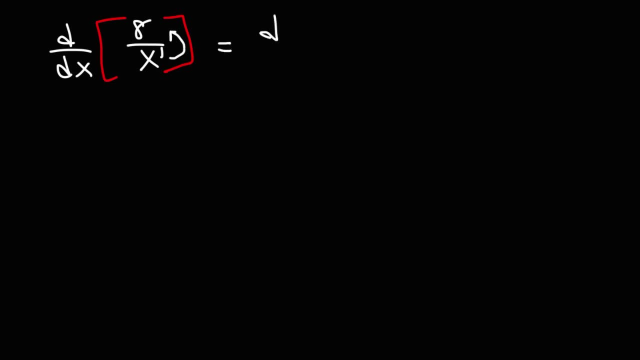 You need to move the x to the top of the fraction. So this is the same as the derivative of 8 times x. So this is the same as the derivative of 8 times x. So this is the same as the derivative of 8 times x raised to the minus 1.. 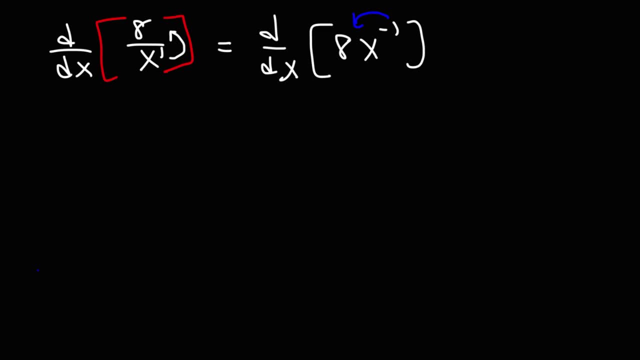 And now we could use the power rule. We can move the exponent to the front, And so it becomes 8 times negative 1, or negative 8. And then x, And then subtract this by 1.. Negative 1 minus 1 is negative 2.. 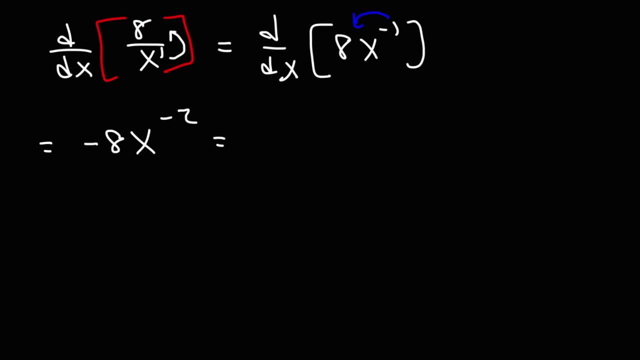 So this is the answer. but we want to get rid of the negative exponents. So what we're going to do is we're going to move x back to the bottom And the negative exponent is going to become positive, So we're going to get negative 1.. 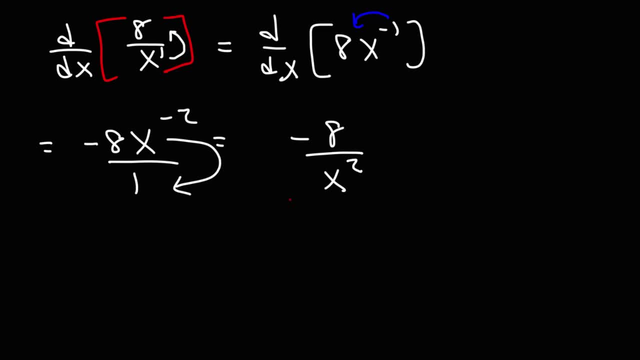 So we're going to get negative 8 over x squared. So this is the final answer for this example. Let's try a similar example. Let's find the derivative of 7 over x squared. Feel free to pause the video if you want to try that problem. 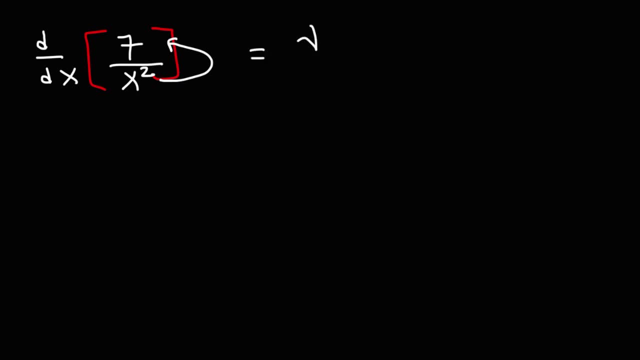 So let's begin by rewriting the expression. So this is equivalent to saying the derivative of 7 times x: x to the minus 2.. Now we could use the power rule, So it's going to be 7 times the derivative of this thing. 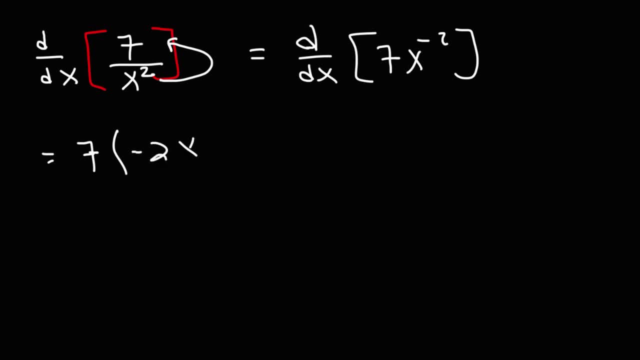 The derivative of x to the minus 2 is negative 2x, And then if you subtract negative 2 by 1, you're going to get negative 3.. Next we can multiply 7 and negative 2. That's negative 14.. 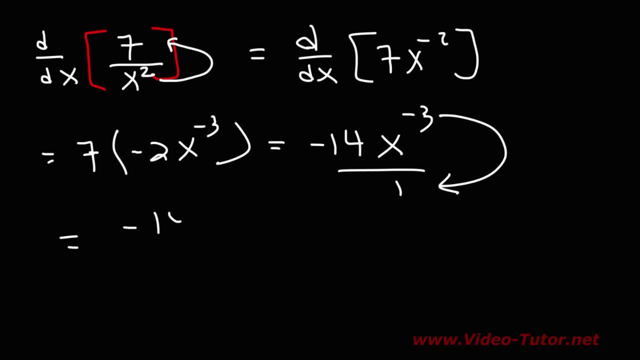 And then we're going to move the negative 3 to the bottom. So the answer is going to be negative: 14 over x, squared, x cubed. Here's another one. Let's find the derivative of 8 over x to the third power. 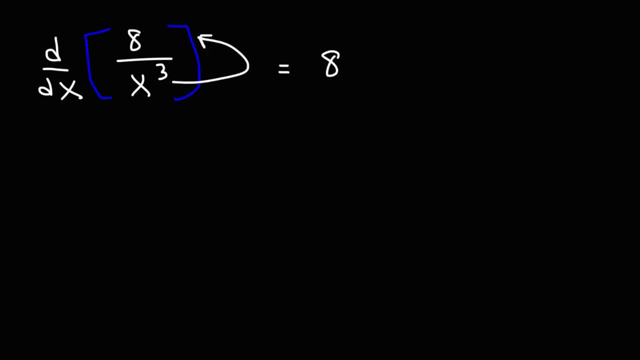 So once again, let's rewrite the expression. So this is the same as finding the derivative of 8x to the minus 3.. Now the derivative of x to the minus 3 is going to be negative 3 times x raised to the negative 4.. 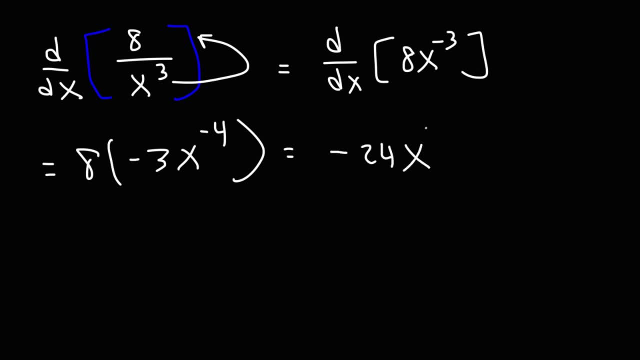 And then 8 times negative, 3 is negative 24.. Now, moving the x variable to the bottom, this is going to give us the final answer: negative 24 over x to the fourth power. Now, what about this problem? What is the derivative? 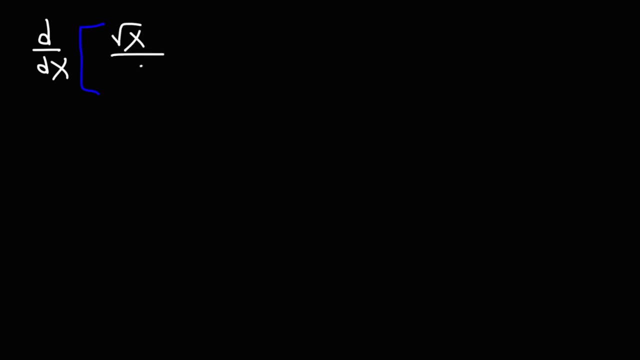 The derivative of, let's say, the square root of x over 5.. So what would you do if you have a square root in the numerator of a fraction? Well, first we want to rewrite the expression. This is the same as the derivative of 1 over 5 times. the square root of x is the same as x to the 1 half. 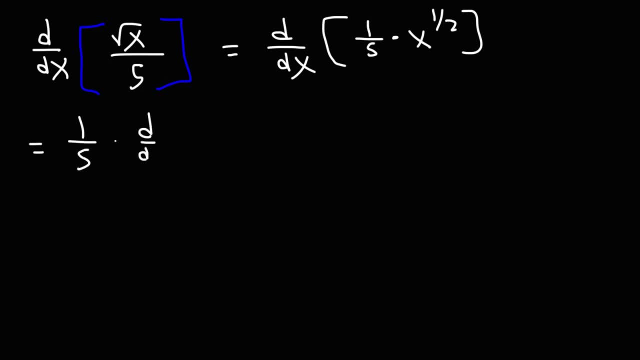 So that's going to be 1 over 5 times the derivative. So that's going to be 1 over 5 times the square root of x to the 1 half. Now let's use the power rule First. we're going to move this to the front. 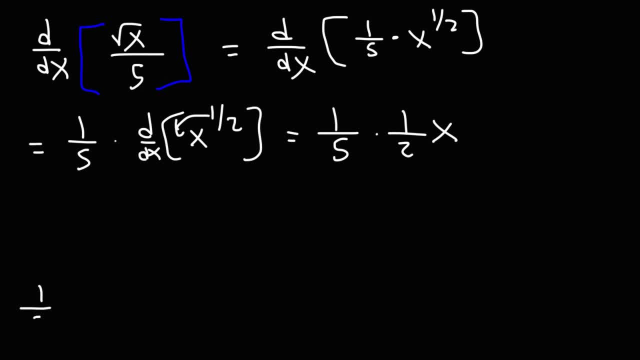 And then we're going to subtract 1 half by 1.. So 1 half minus 1, we could change the negative 1 to 2 over 2 to get common denominators, And then 1 minus 2 is negative 1.. 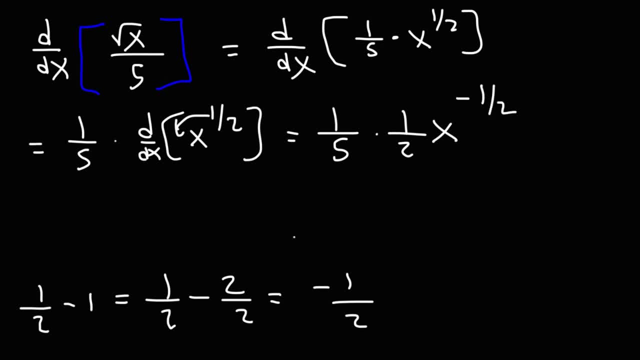 So 1 half minus 1 is negative 1 half. And now we can multiply 1 over 5 by 1 over 2. So 5 times 2 is negative 1. So 5 times 2 is 10.. 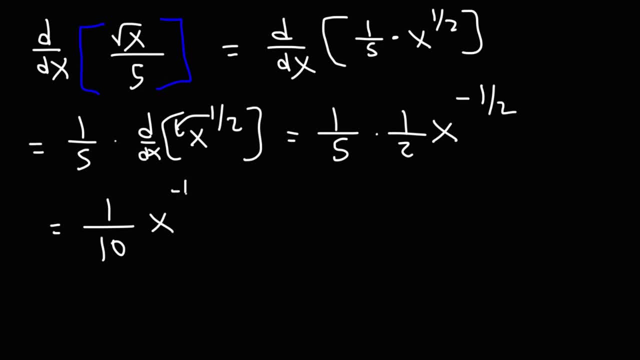 So we're going to get 1 over 10, x to the minus 1 half, Which you can write that as x to the negative, 1 half over 10.. You can just multiply those two together. Now we want to get rid of the negative exponent. 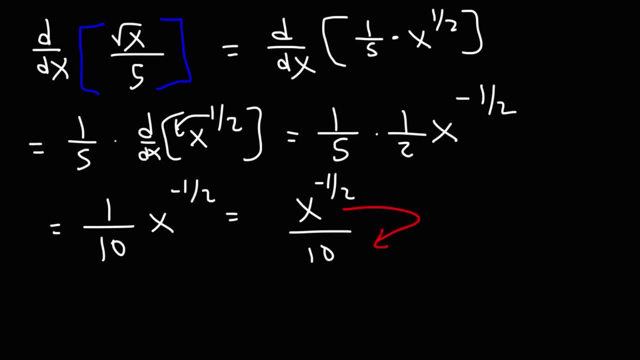 To do that, we need to move the variable x to the bottom. So our answer is 1 over 10, x to the 1 half. Now, even though this is the correct answer, it's not in its most simplified form Because we need to convert it back. 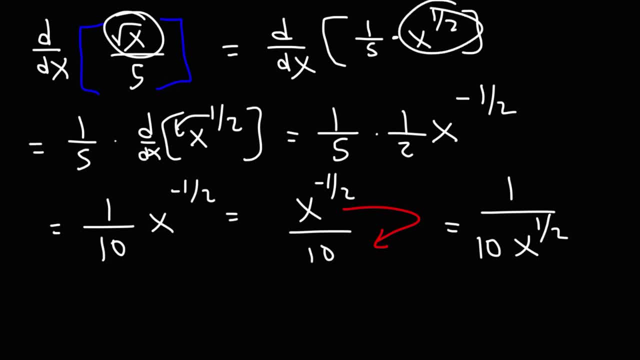 To its radical form. Keep in mind: x to the 1 half is equivalent to the square root of x. So we can write our final answer as: 1 over 10 square root of x. Now you can rationalize this answer, but I'm going to leave it like this. 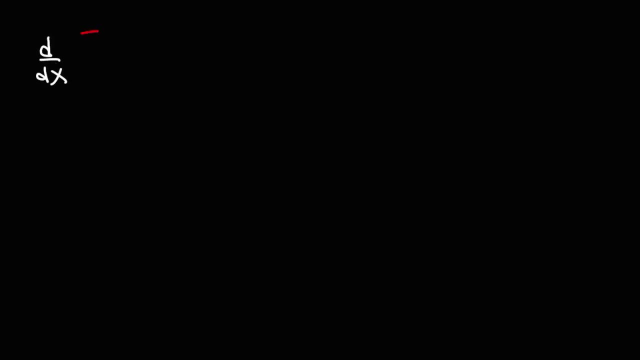 Now let's work on a similar but slightly different problem. So in this example we're going to find the derivative of 7 divided by the square root of x. Feel free to take a minute to try this And let's start that problem. 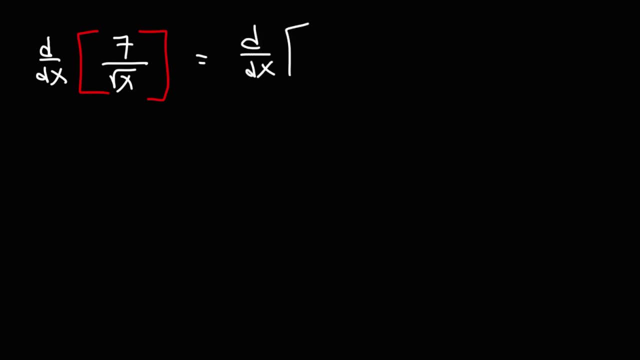 So the first thing we're going to do is we're going to rewrite the problem. The square root of x is the same as x to the 1 half. Next, we'll need to move the x variable to the top before we can use the product rule. 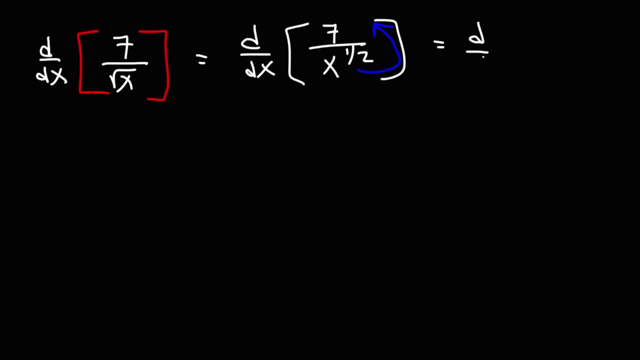 I mean not the product rule but the power rule. So we have the derivative of 7 times x to the negative 1 half. So now we're going to move the negative 1 half to the front And then Subtract negative 1 half by 1.. 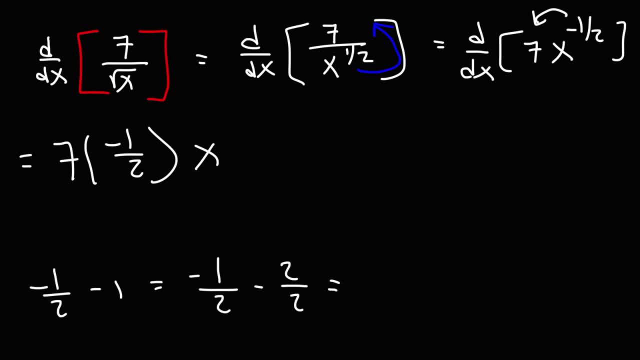 Let's change negative 1 to negative 2 over 2, just like we did before, And now negative 1 minus 2 is negative 3.. So negative 1 half minus 1 is negative 3 over 2.. Now let's see if we can combine this answer into a single fraction. 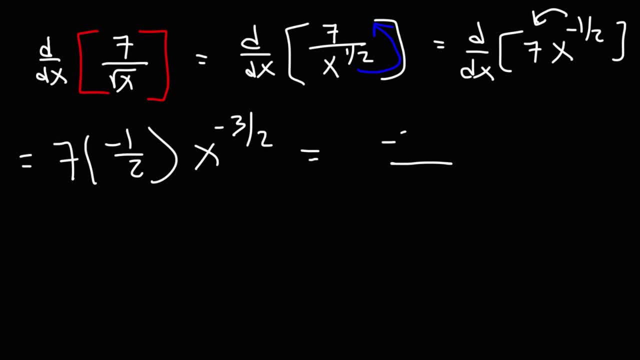 The 7 and the negative sign are on top of the fraction. The 2 is on the bottom And since this fraction is multiplied by x, it's automatically going to put the x on top. Now the next thing we need to do is get rid of the negative exponent by moving the x variable back to the bottom. 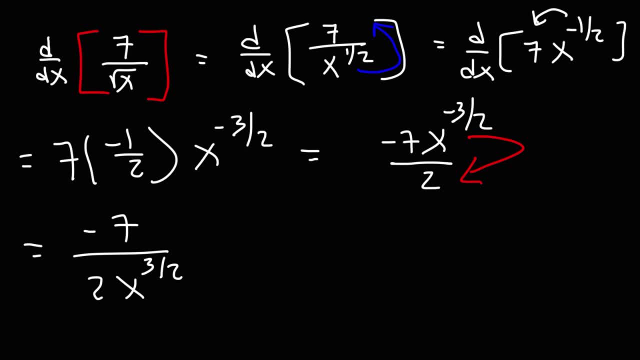 So this is what we now have. Next, what we can do is get rid of. we can convert this back into its radical form, But it's important to understand that x to the 3 half can be rewritten as x to the 1 half. 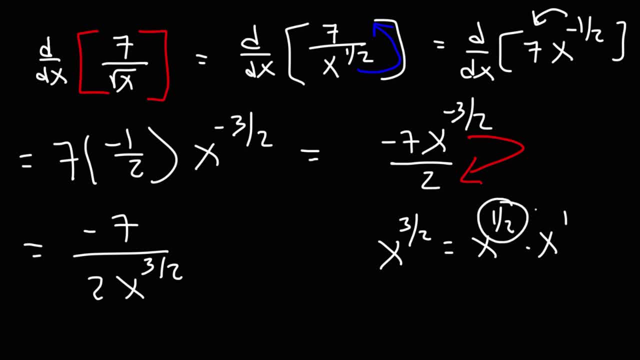 Times x to the first power, Because a half plus 1 is 3 halves, Or 0.5 plus 1 is 3 over 2, which is 1.5.. And x to the 1 half is equal to the square root of x. 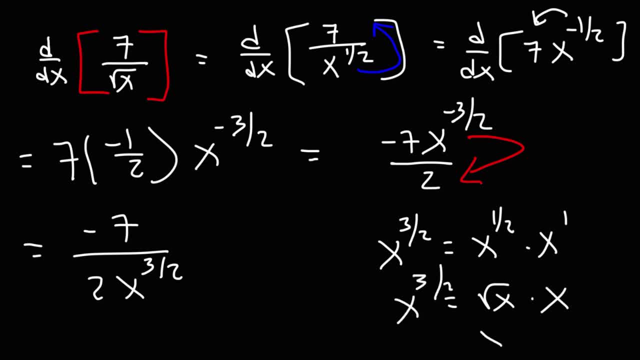 So we can replace x to the 3 half with x root x. So we can write the final answer as negative 7, 2.. x times the square root of x. So that's it for this problem. Now let's work on one more problem. 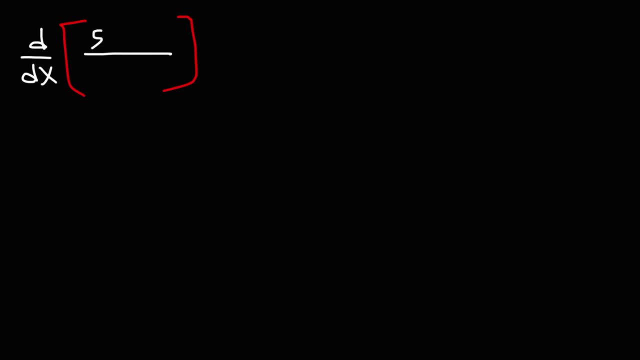 Go ahead and find the derivative of this fraction, 5 plus 3, x divided by x squared plus 7.. Now, for problems like this, you need to use something called the quotient rule, And here's the formula for that: The derivative of a fraction f over g. 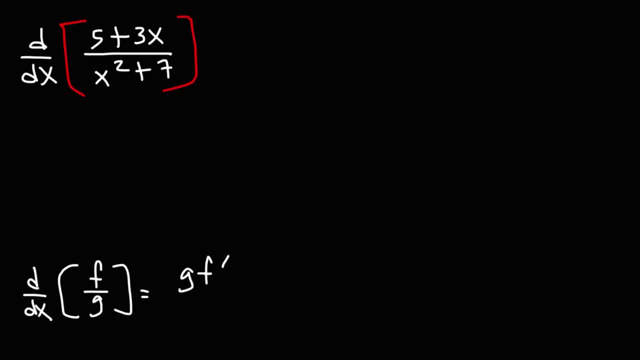 That's going to be equal to g, f prime minus f, g prime over g squared. Some books would use the variables u and v, So in this case we need to define what f and what g is. So f is the stuff on the numerator. 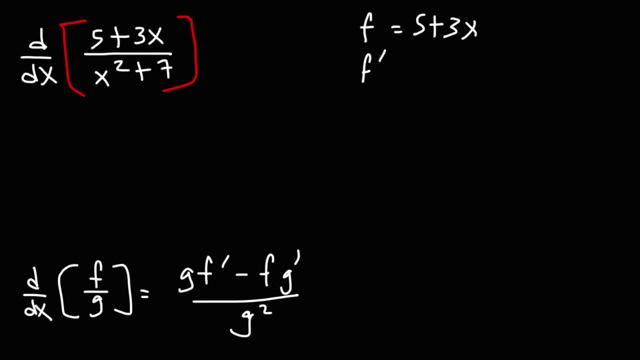 That's 5 plus 3 x. f prime Is the derivative of that expression. The derivative of a constant is 0.. And the derivative of 3 x is just 3.. Now g is the function on the bottom, It's the stuff in the denominator of the fraction. 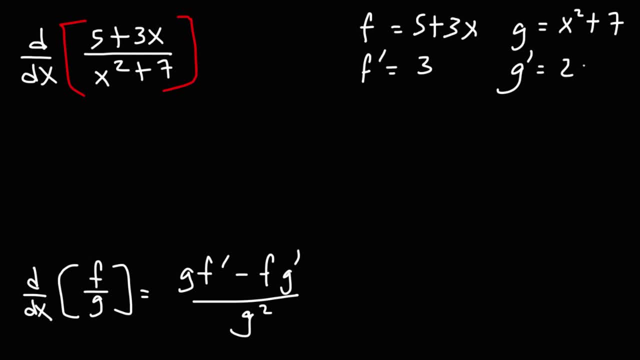 To find g prime, we need to find the derivative of x squared, which is 2x, And the derivative of 7 is 0.. So now we just got to plug everything in to this formula. So it's g which is x squared plus 7.. 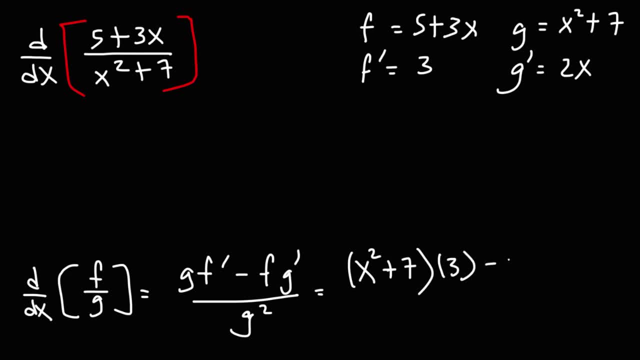 Times f prime, which is 3.. Minus f, which is 5 plus 3x Times g prime, which is 2x Divided by g squared, So that's x squared plus 7 squared. So at this point we can get rid of this information. 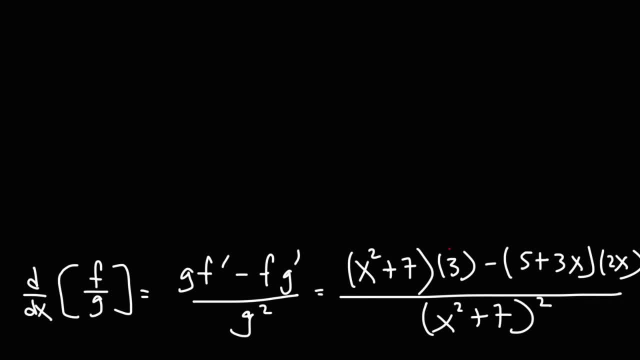 And now we just got to simplify this expression, So let's distribute the 3.. So first we're going to have 3x squared, And then 3 times 7 is 21.. Next, we're going to have 3x squared. 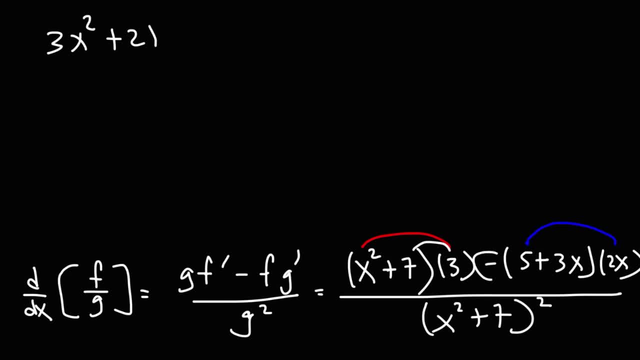 Next we're going to have 2x times 5, which is 10x, But we have a negative sign in front of that, So that's going to be negative 10x, And then 2x times 3x, that's 6x squared.